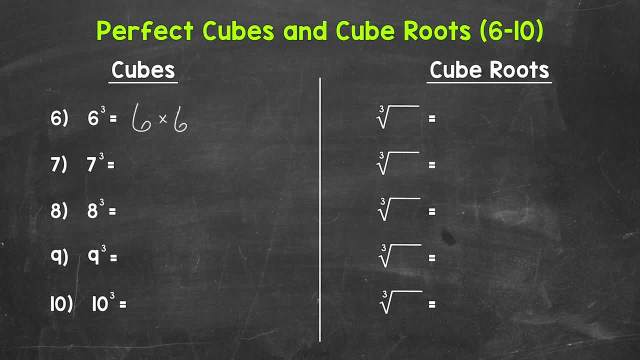 That means 6 times 6 times 6.. 6 times 6 is 36 times 6 equals 216.. 6 cubed equals 216. That means that the cube root of 216 equals 6.. Let's move on to number 7, where we have 7 cubed. 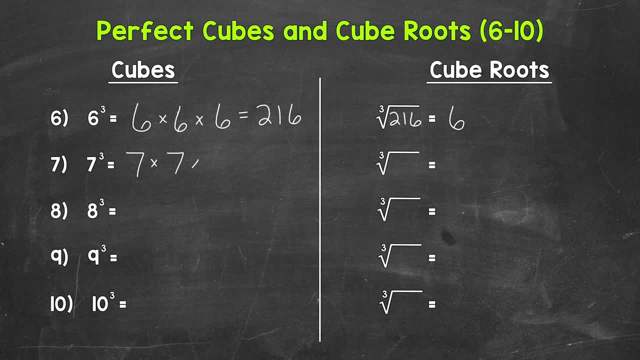 That means 7 times 7 times 7.. 7 times 7 is 49 times 7 equals 346.. 7 cubed equals 343.. 7 cubed equals 343.. That means that the cube root of 343 equals 7.. 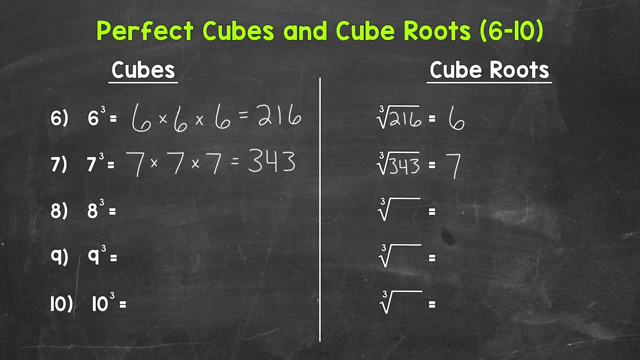 Let's move on to number 8, where we have 8 cubed. That means 8 times 8 times 8.. 8 times 8 is 64.. 64 times 8 equals 512.. 8 cubed equals 512.. 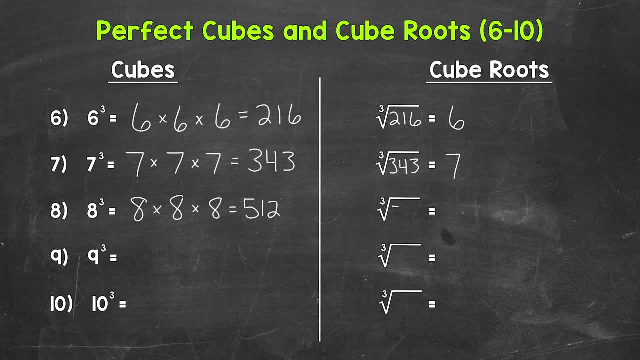 That means that the cube root of 512 equals 8.. Let's move on to number 9,, where we have 9 cubed. That means 9 times 9 times 9.. 9 times 9 is 81.. 81 times 9 equals 729. 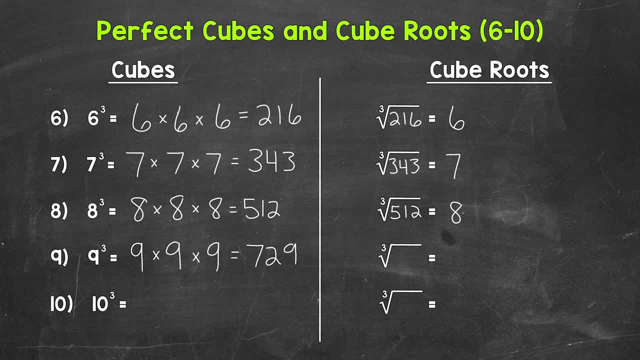 So 9 cubed equals 729.. That means that the cube root of 729 equals 9.. Let's move on to number 10, where we have 10 cubed. That means 10 times 10 times 10.. 10 times 10 is 100. 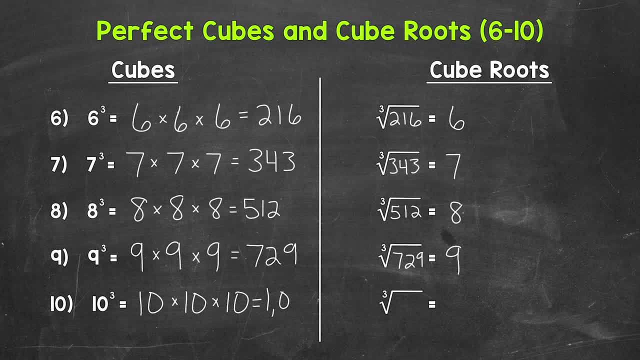 100 times 10 equals 1000.. 10 cubed equals 1000.. That means that the cube root of 1000 equals 10.. So there you have it. There are the 6th through 10th perfect cubes and cube roots.